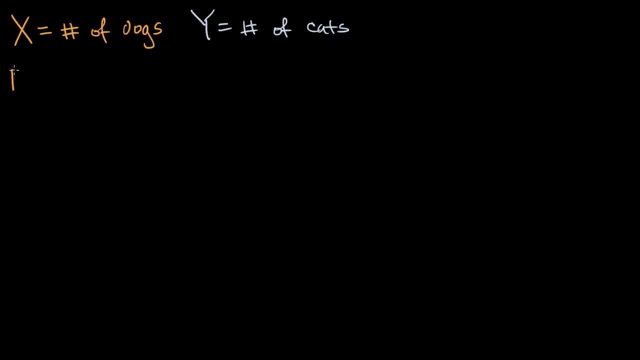 of each of these random variables are the expected value, So the expected value of x, which I could also denote as the mean of our random variable x. let's say, I expect to see three dogs a day And similarly for the cats, the expected value of y. 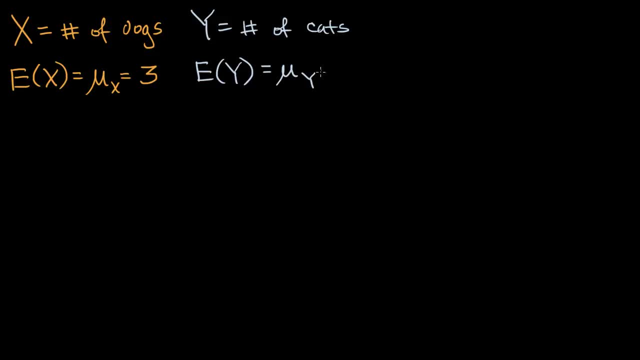 is equal to. I could also denote that as the mean of y is going to be equal to, and this is just for the sake of argument. let's say, I expect to see four cats a day And in previous videos we defined: how do you take? 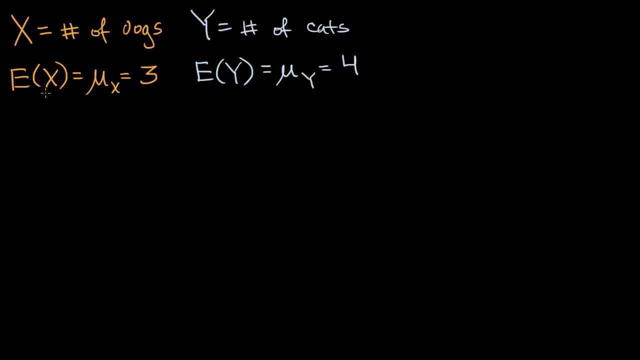 the mean of a random variable or the expected value of a random variable. What we're going to think about now is what would be the expected value of x plus y, Or, another way of saying that, the mean of the sum of these two random variables. 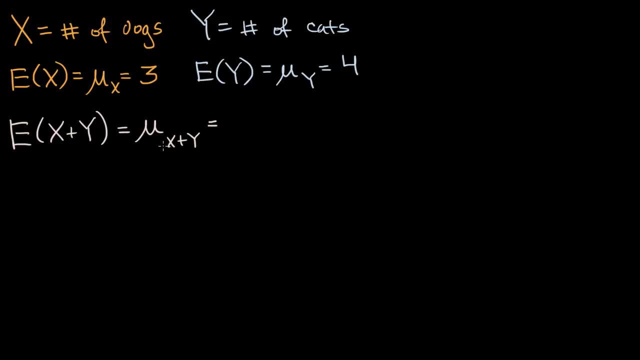 Well, it turns out- and I'm not proving it just yet- that the mean of the sum of random variables is equal to the sum of the means. So this is going to be equal to the mean of random variable x plus the mean of random variable y. 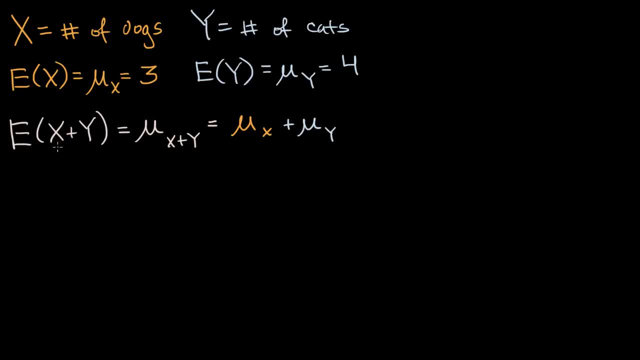 And so, in this particular case, if I were to say, well, what's the expected number of dogs and cats that I would see in a given day? Well, I would add these two means It would be three plus four, It would be equal to seven. 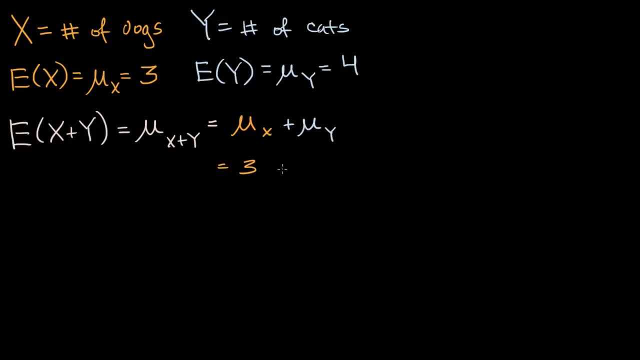 So, in this particular case, it is equal to three plus four, which is equal to, which is equal to seven. And similarly, if I were to ask you the difference, if I were to say: well, what's the? how many more cats in a given day? 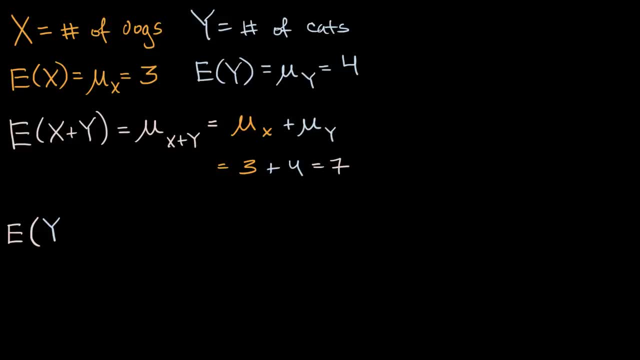 would I expect to see than dogs. So the expected value of y minus x, What would that be? Well, intuitively, you might say: well, hey, if we can add random, if the expected value of the sum is the sum of the expected values. 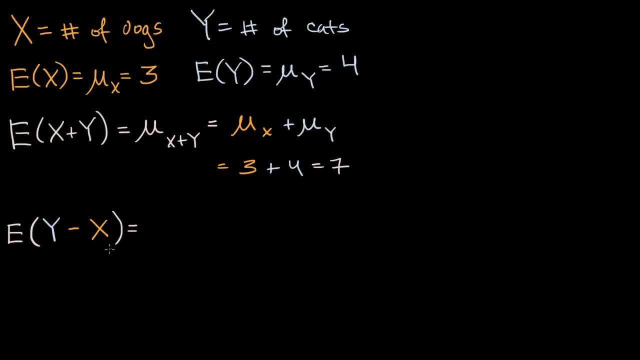 then the expected value or the mean of the difference will be the differences of the means, And that is absolutely true. So this is the same thing as the mean of y minus x, which is equal to the mean of y. It's going to be equal to the mean of y.